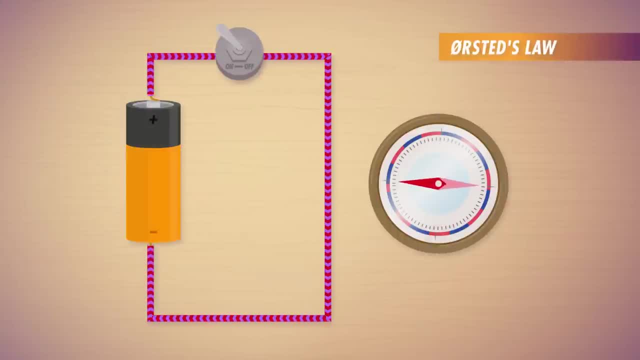 He turns on the current that runs through the wire and he notices that the needle in the compass starts to move. And when he turns the current off, the needle moves back to where it was. Then he runs the current through the wire in the opposite direction and sees the needle move the other way. 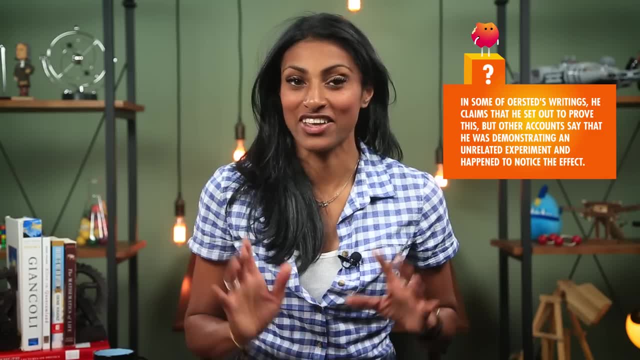 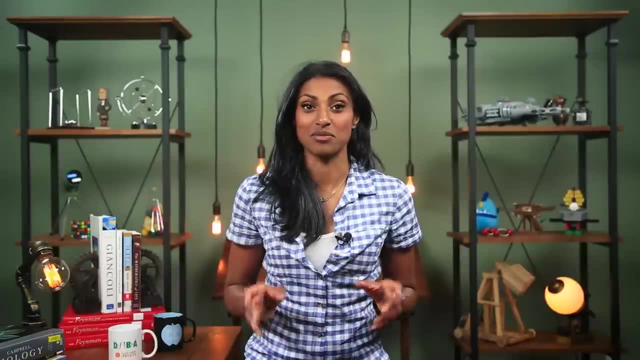 What Ørsted demonstrated that day was a fundamental discovery – the connection between electricity and magnetism, And it changed the field of physics forever. The relationship between electricity and magnetism not only explains what Ørsted and his students witnessed in 1820,. 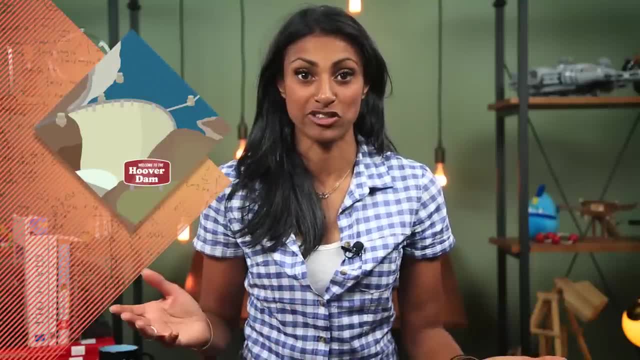 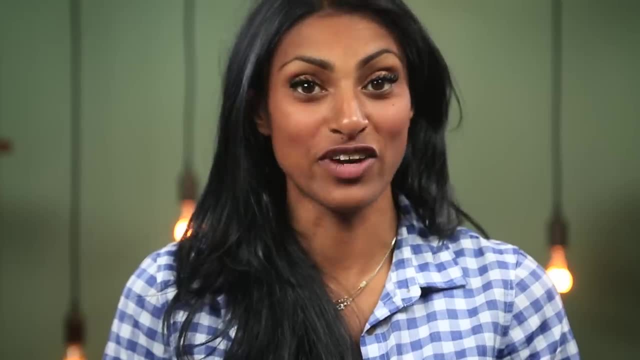 it also makes possible much of the technology that's used today, from hydroelectric dams to your smartphone. It even explains why Earth's magnetic field is essentially keeping you from being cooked alive right now, And all you really need to understand the basics of magnetism and electricity is this: 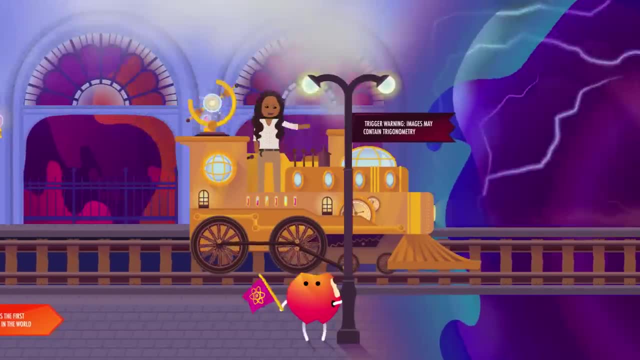 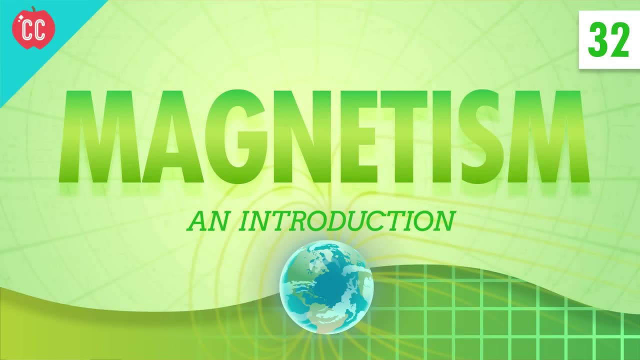 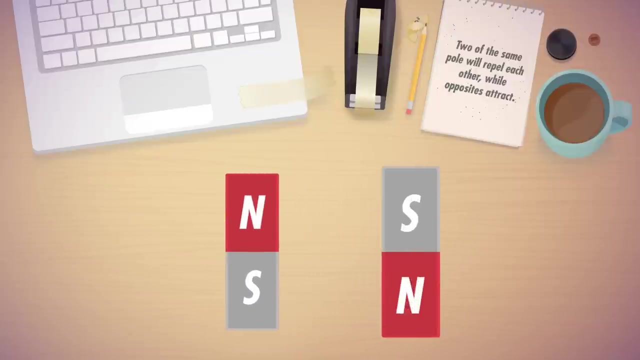 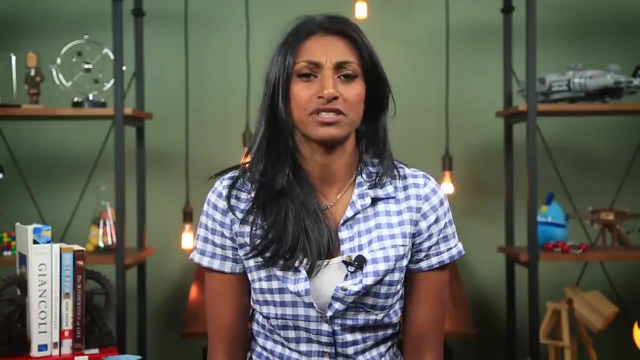 You're probably familiar with the basics of magnets already. They have a North and South pole. two of the same pole will repel each other, while opposites attract. Only certain materials, especially those that contain iron, can be magnets. It depends on their molecular properties. 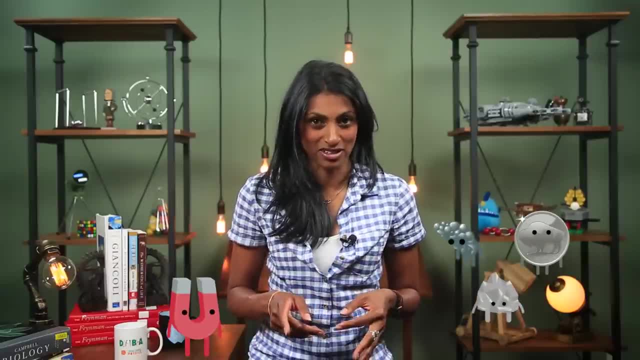 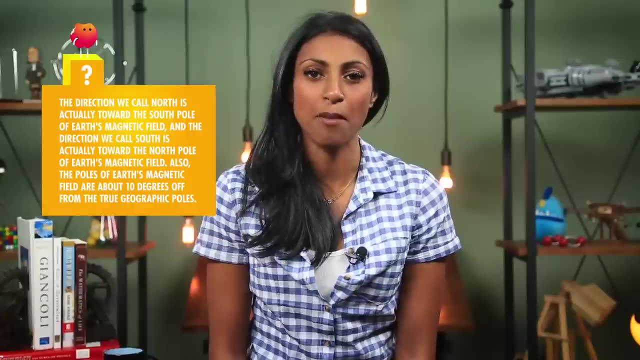 And other metals, including cobalt, nickel and iron, are attracted to magnets, Even though they aren't magnets. They're magnets themselves, like the metal in your refrigerator door, And there's a magnetic field around Earth, which is why you can use a compass to figure out which way is North. 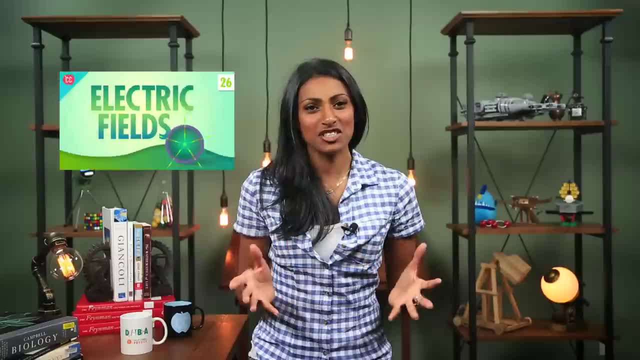 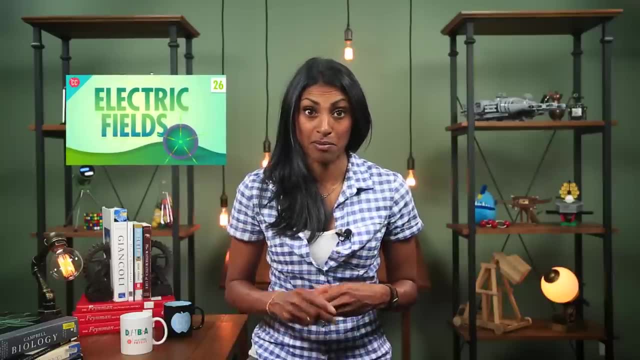 The magnet in the compass aligns itself with the Earth's magnetic field. Just as we use electric field lines to represent the electric field created by charges, we can draw magnetic field lines to represent magnetic fields created by magnets. And, as with electric fields, the more crowded the lines are, the stronger the magnetic field. 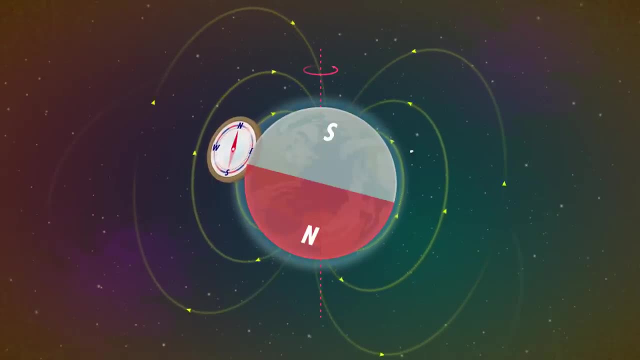 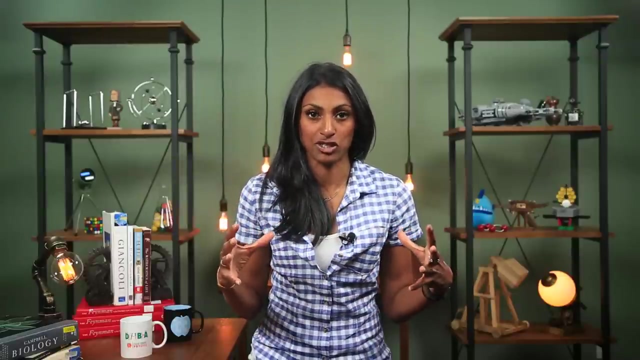 The lines point from the North pole to the South pole, like how electric field lines point from the positive to the negative. But there's a key difference: You can have an electric field spreading outward from a single electric charge, But that can't happen with magnets, because you can't isolate one magnetic pole. 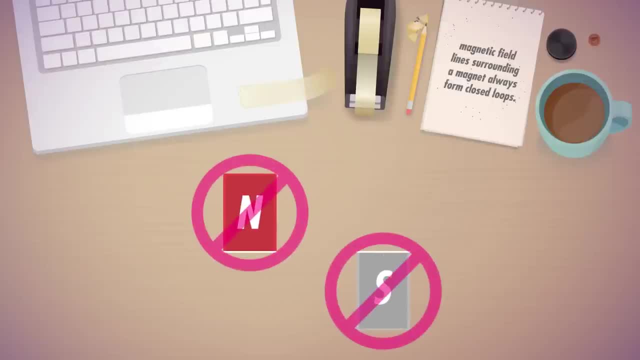 If you chop a bar magnet in half, you don't end up with one North magnet and one South magnet. You end up with two magnets, each with its own North pole and South pole. This means that the magnetic field lines surrounding a magnet always form closed loops. 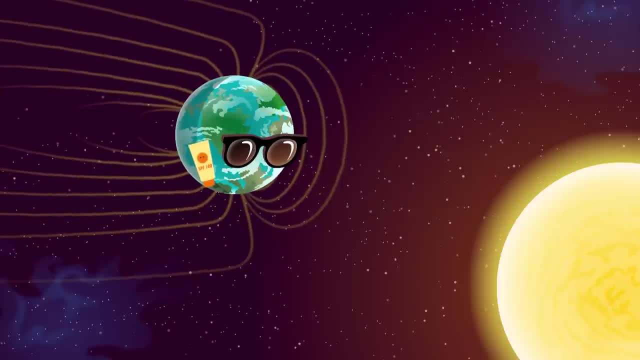 It even explains why Earth's magnetic field is essentially keeping you from being cooked alive right now. 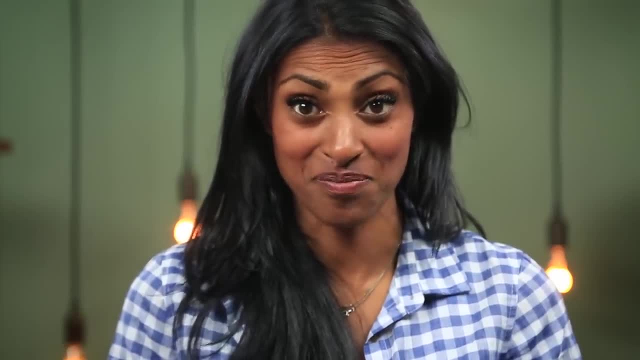 And all you really need to understand the basics of magnetism and electricity is this. You're probably familiar with the basics of magnets already. They have a north and south pole – two of the same pole will repel each other, while opposites attract. Only certain materials, especially those that contain iron, can be magnets. It depends on their molecular properties. And other metals, including cobalt, nickel, and iron, are attracted to magnets, even though they aren't magnets themselves, like the metal in your refrigerator door. And there's a magnetic field around Earth. Which is why you can use a compass to figure out which way is north. The magnet in the compass aligns itself with the Earth's magnetic field. Key difference. You can have an electric field spreading outward from a single electric charge. But that can't happen with magnets, because you can't isolate one magnetic pole. If you chop a bar magnet in half, you don't end up with one north magnet and one south magnet. You end up with two magnets, each with its own north pole and south pole. This means that the magnetic field lines surrounding a magnet always form closed loops. We measure magnetic fields using a unit called the Tesla. One Newton per ampere meter and one tesla is a very strong magnetic field. The fields from some of the strongest superconducting magnets in the world are only 10 teslas. 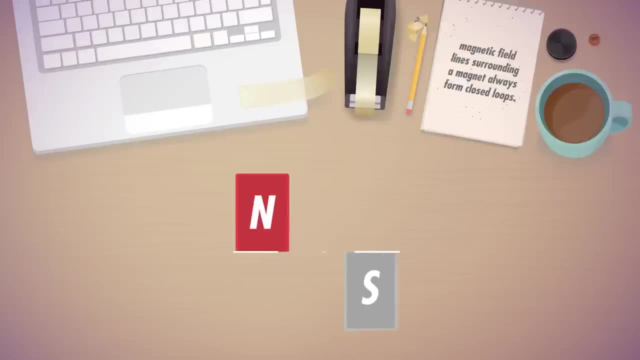 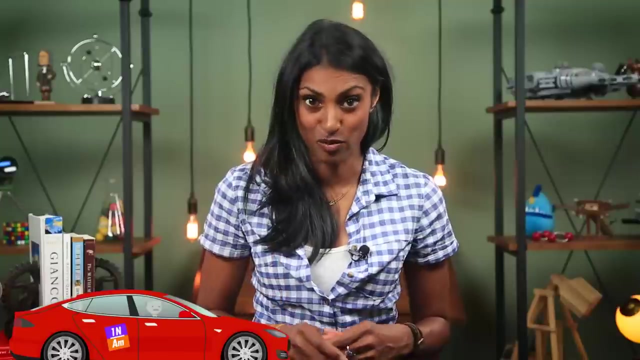 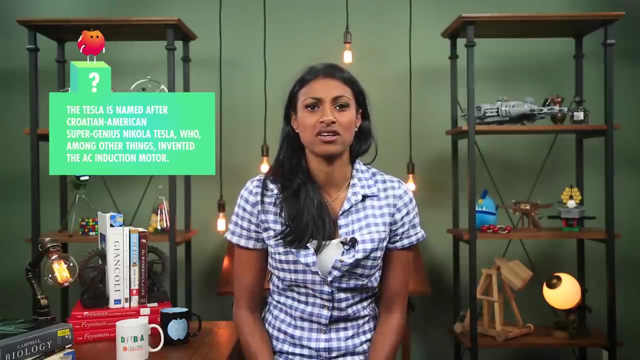 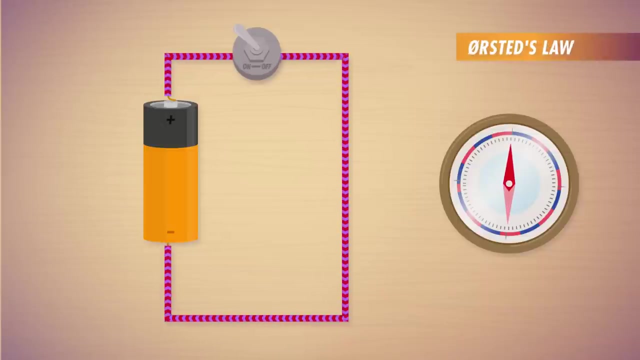 Now, when Ørsted was doing a demonstration on that fateful day in 1820, he was using a regular compass magnet. But when he brought the magnet closer to a wire carrying a current, the magnetic field from the current exerted a force on the needle, moving it to point in a different direction. Ørsted had discovered one of the fundamental principles of electromagnetism. An electric current produces a magnetic field. After several months of experimenting, Ørsted figured out that when a current runs through a wire, the magnetic field that it produces surrounds the wire. Expressed with field lines, the magnetic field would appear as circles with the wire at their center. If the current was coming straight towards you, the field lines would be pointing counterclockwise. And we use the vector b to represent the magnetic field. 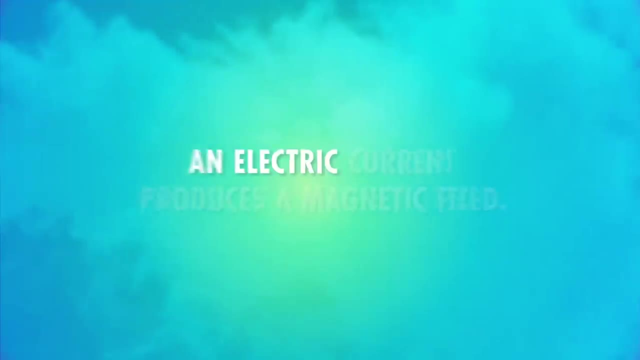 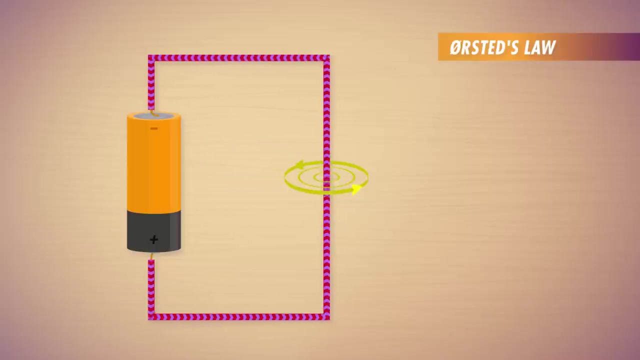 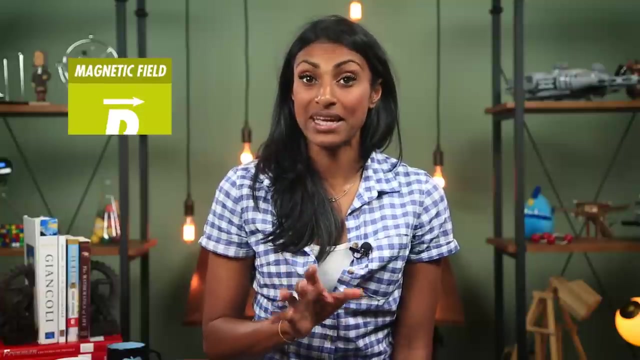 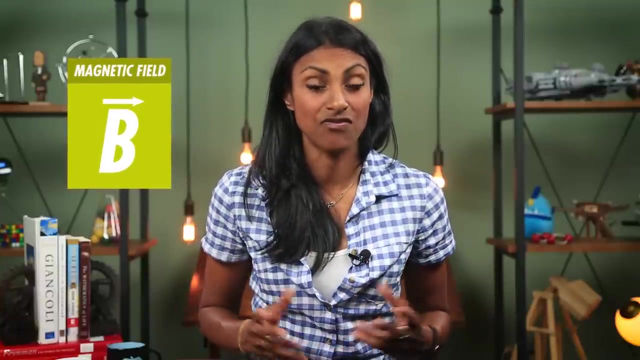 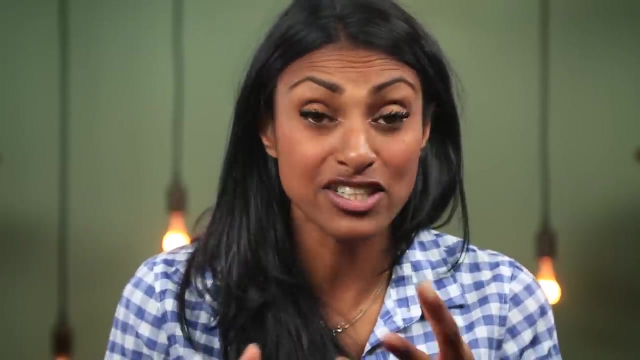 The magnitude of the vector is the strength of the magnetic field, and the direction of the vector is the field's direction. Now, there's an easy way to remember how the direction of the electric current and the direction of the magnetic field work. It's called the first right-hand rule, because there are actually three right-hand rules. Just take your right hand and point your thumb in the direction of the electric current. Now curl your fingers. The direction your fingers are curling, that's the way the magnetic field lines are pointing. And likewise, if you know the direction of the magnetic field lines, you can use the rule to figure out the direction of the current in the wire. It really comes in, uh, handy. Now, if a current running through a wire exerts a force on a magnet, you might expect the opposite to be true. 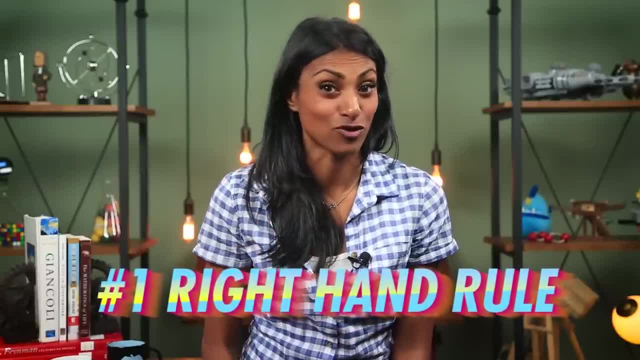 That a magnet exerts a force on a current running through a wire. And it does! Which is good, because that's what's protecting us from harmful radiation from the Sun right now. 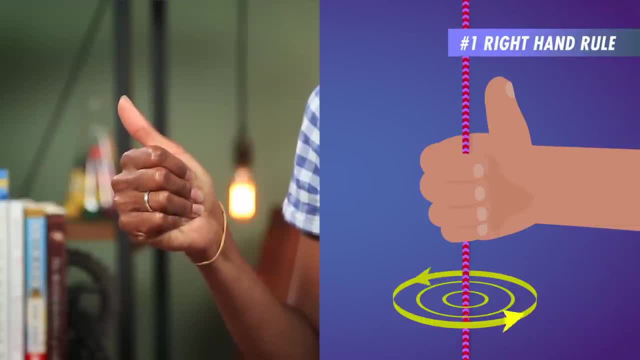 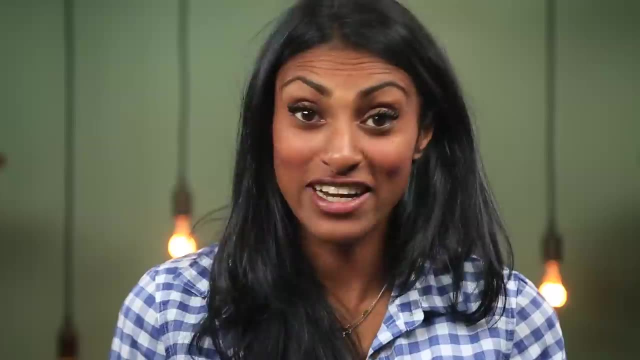 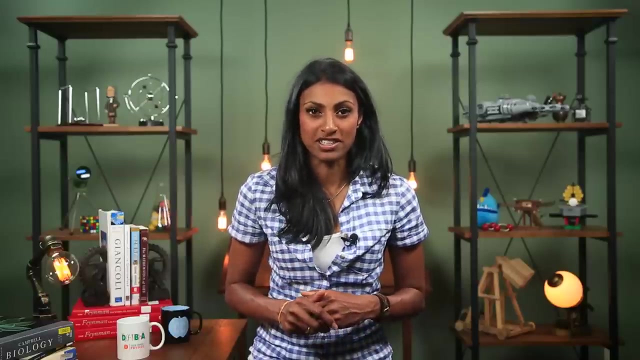 The direction of the force from a magnetic field on a current running through a wire will be perpendicular to both the magnetic field and the current. Which brings us to the second right-hand rule. This one helps you keep track of three directions – the direction of the magnetic field, the current, and the force. Here's how to use the second right-hand rule. Point your arm in the direction of the current. Then bend your fingers. 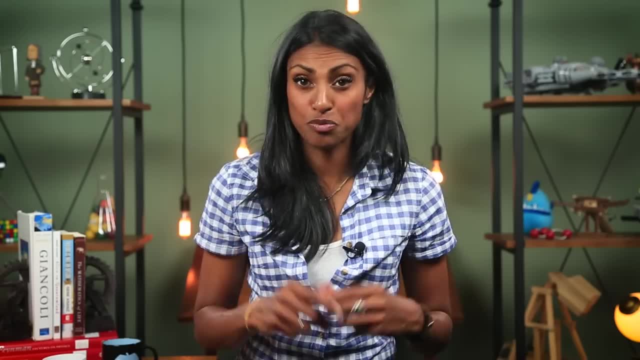 So they're perpendicular to your palm. This represents the direction of the magnetic field. 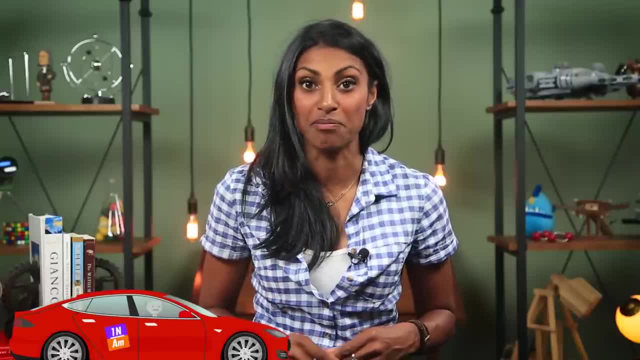 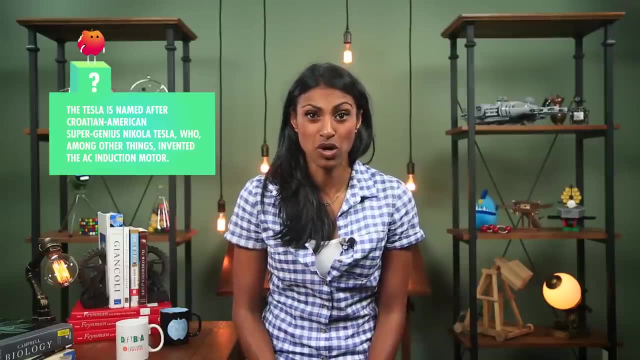 We measure magnetic fields using a unit called the tesla, which is one newton per ampere meter, And one tesla is a very strong magnet. The magnetic field that fills from some of the strongest superconducting magnets in the world are only ten teslas. 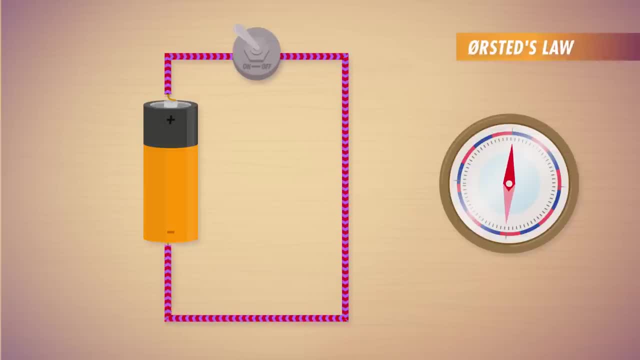 Now, when Ørsted was doing a demonstration on that fateful day in 1820, he was using a regular compass magnet. But when he brought the magnet closer to a wire carrying a current, the magnetic field from the current exerted a force on the needle, moving it to point in a different direction. 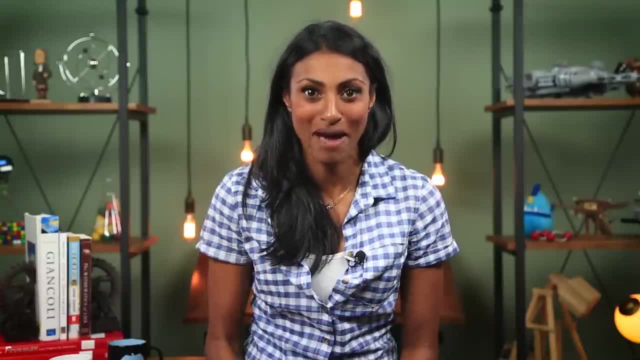 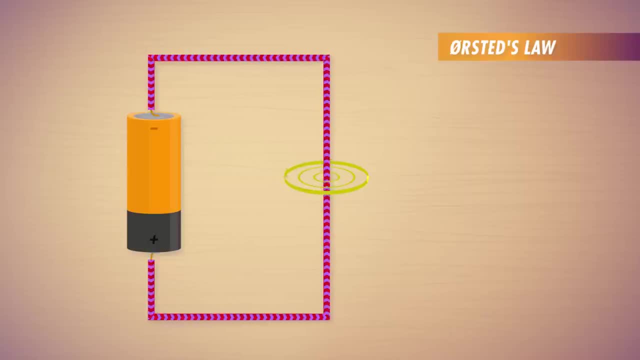 Ørsted had discovered one of the fundamental principles of electromagnetism: An electric current produces a magnetic field. After a few more months of experimenting, Ørsted figured out that when a current runs through a wire, the magnetic field that it produces surrounds the wire. 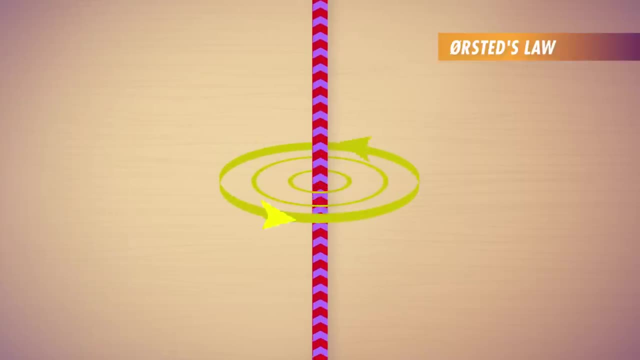 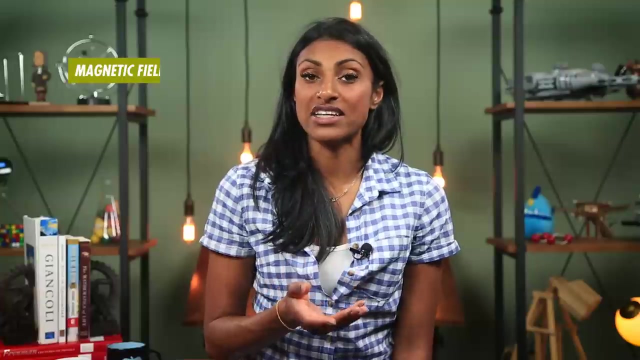 Expressed with field lines. the magnetic field would appear as circles with the wire at their center. If the current was coming straight towards you, the field lines would be pointing counterclockwise, And we use the vector b to represent the magnetic field. 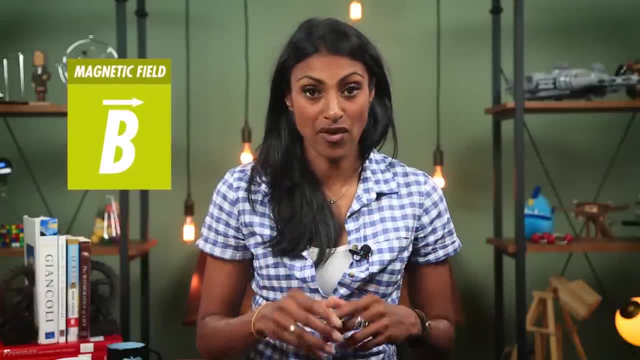 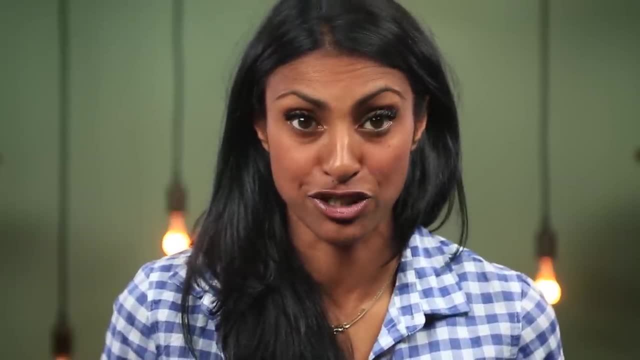 The magnitude of the vector is the strength of the magnetic field, and the direction of the vector is the field's direction. Now there's an easy way to remember how the direction of the electric current and the direction of the magnetic field it produces relate to each other. 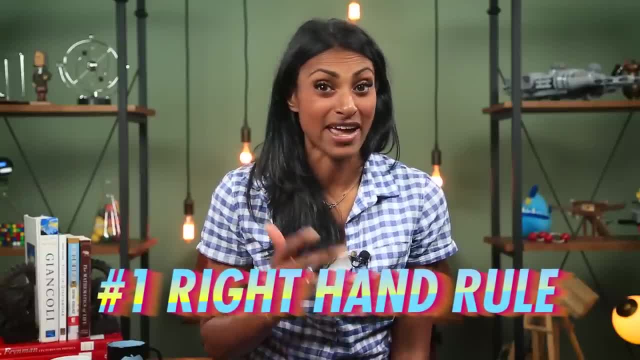 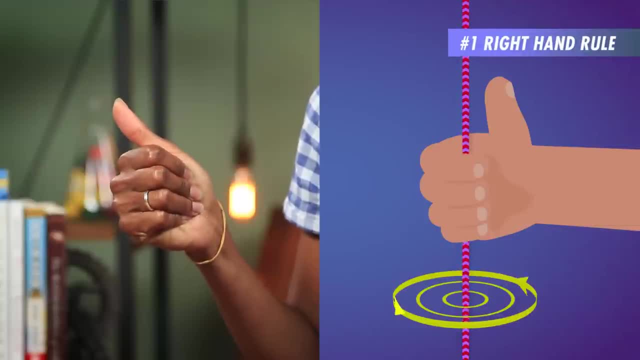 It's called the first right-hand rule because there are actually three right-hand rules. Just take your right hand and point your thumb in the direction of the electric current. Now curl your fingers The direction your fingers are curling. that's the way the magnetic field lines are pointing. 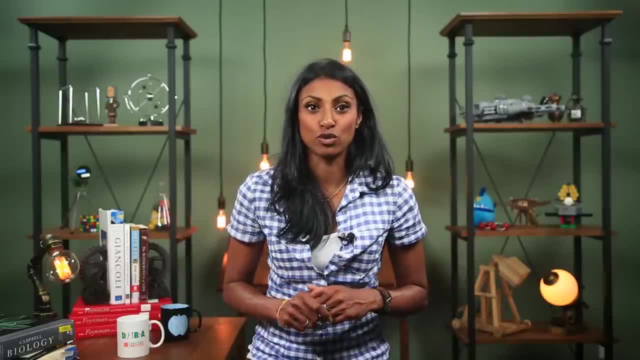 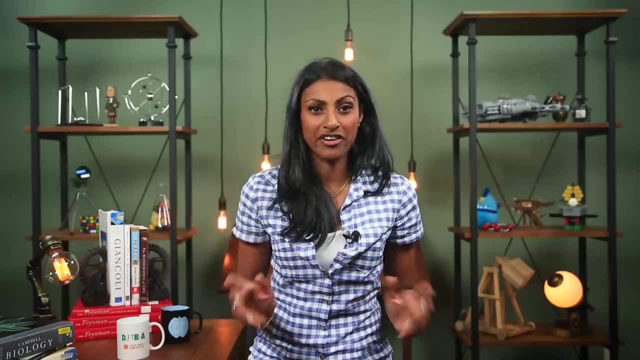 And likewise, if you know the direction of the magnetic field lines, you can use the rule to figure out the direction of the current in the wire. It really comes in uh handy. Now, if a current running through a wire exerts a force on a magnet, you might expect the opposite to be true as well. 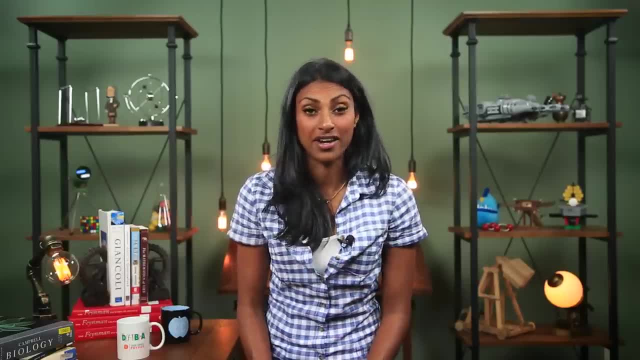 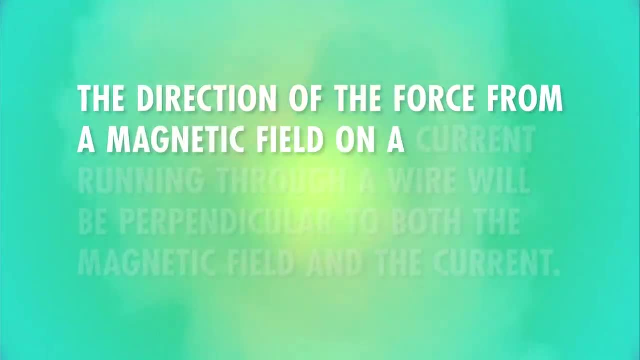 That a magnet exerts a force on a magnet, That a force on a current running through a wire, And it does, Which is good, because that's what's protecting us from harmful radiation from the Sun right now. The direction of the force from a magnetic field on a current running through a wire will be perpendicular to both the magnetic field and the current. 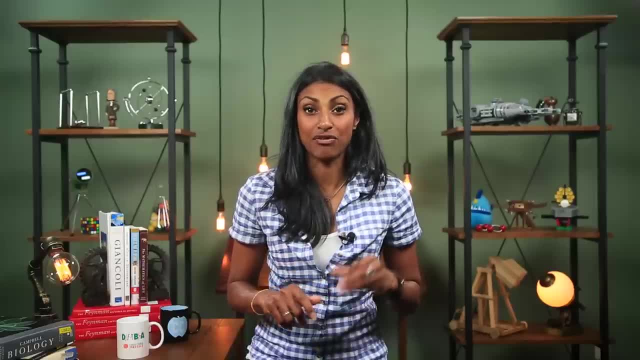 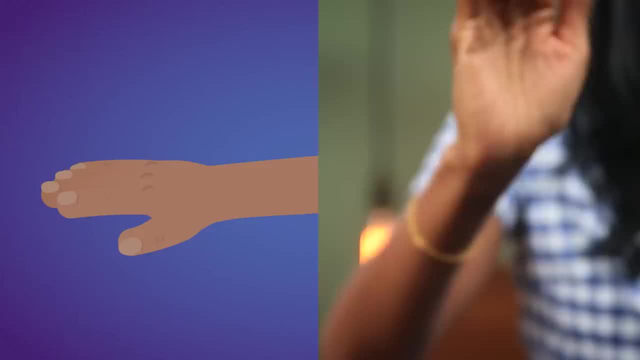 Which brings us to the second right-hand rule. This one helps you keep track of three directions – the direction of the magnetic field, the current and the force. Here's how to use the second right-hand rule: Point your arm in the direction of the current, then bend your fingers so they're perpendicular to your palm. 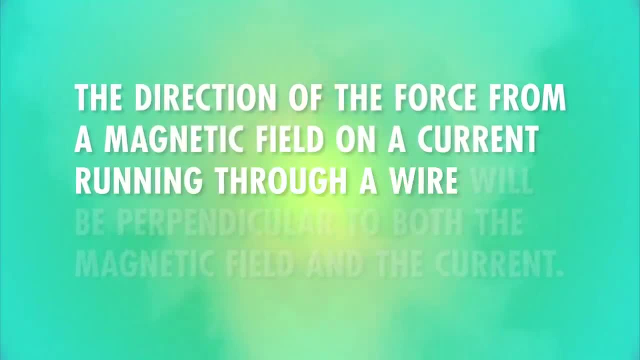 Your thumb, which is perpendicular to your fingers, is the direction of the force on the wire. But what about the strength of that force? 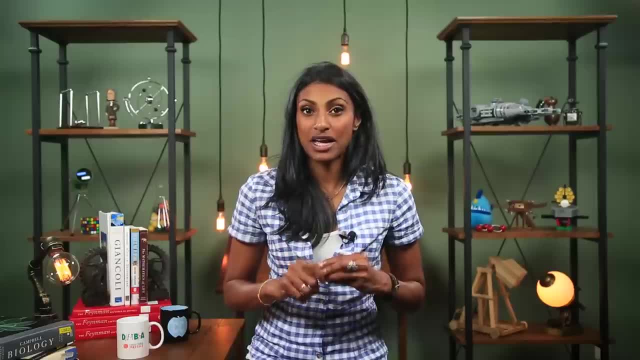 You can use your hands to figure this out, too. But you'll have to use them to do math. Sorry. 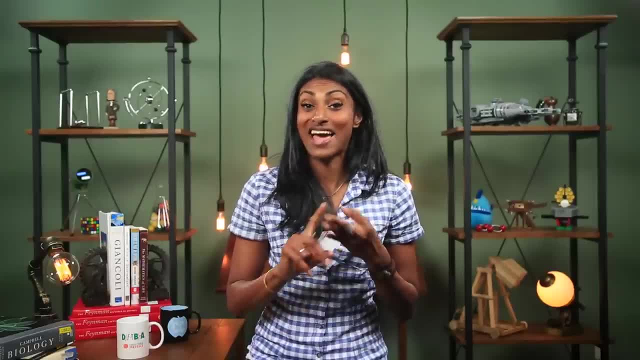 The magnitude of the force from a magnetic field on a wire is equal to ilb sine theta. This equation tells us that there are four factors that affect the magnitude of the force. First, there's the current in the wire. 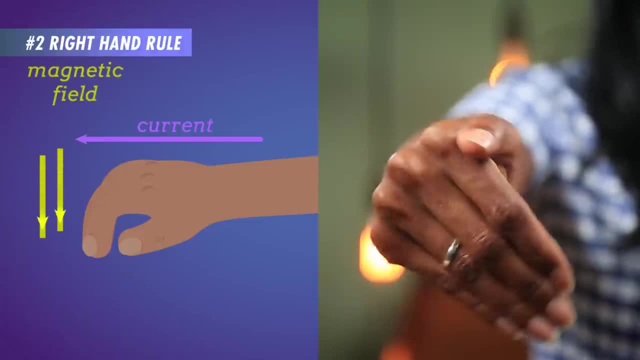 That's I. And the stronger it is, the stronger the force is. 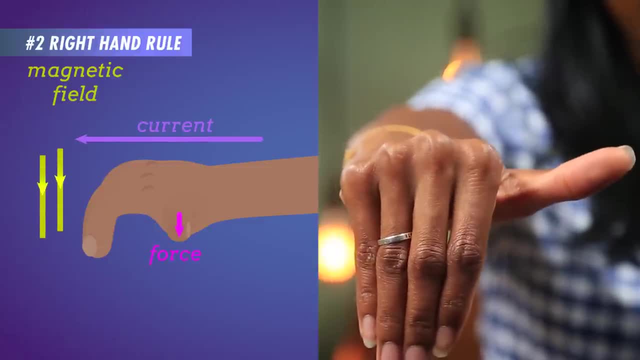 Second, there's the length of the wire running through the magnetic field. That's l. And the longer the wire is, the stronger the force is. 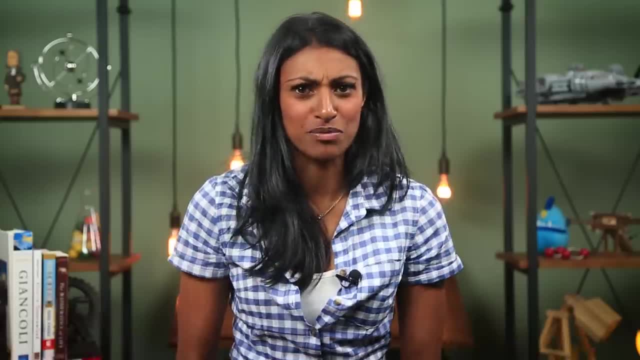 Third, there's the magnetic field B. And the stronger B is, the stronger the force. 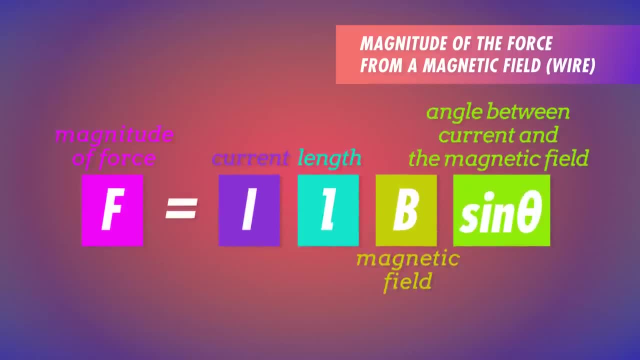 Finally, the closer to perpendicular the current is with respect to the magnetic field's direction, the stronger the force is. 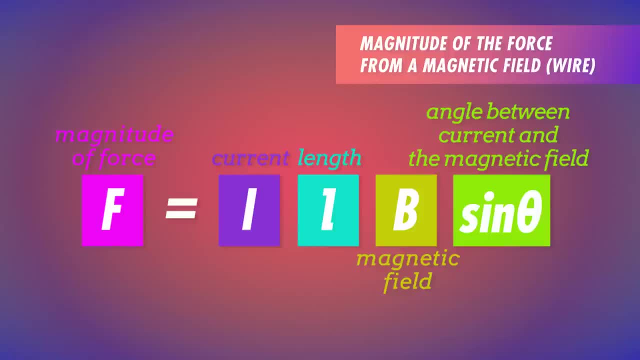 That's where sine theta comes in. Its maximum value is 1 when theta is 90 degrees. 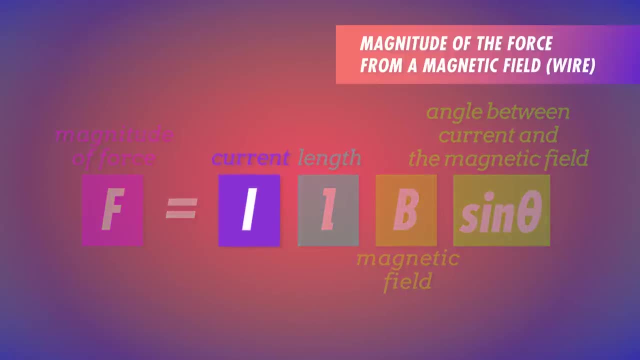 So the current is perpendicular to the magnetic field lines. That's when the force will be stronger. 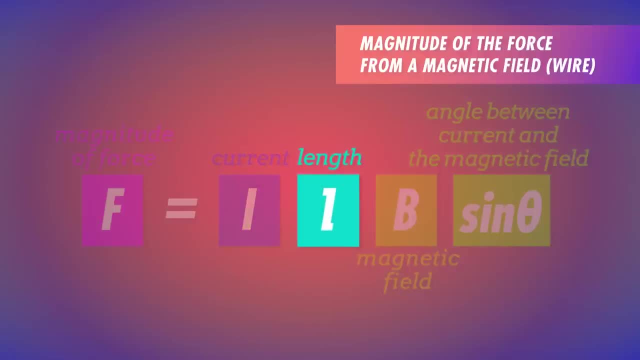 Similarly, the minimum value of sine theta is zero when theta is zero. So that means the current is parallel to the magnetic field lines, and in that case, there won't be any force on the wire at all. 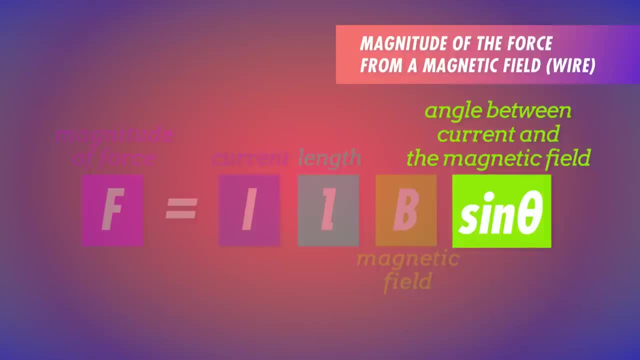 Now, all of this math can help us understand how we're being protected right now from solar radiation. The Sun is constantly shooting radiation towards Earth in the form of charged particles. But luckily for us, Earth has a magnetic field. 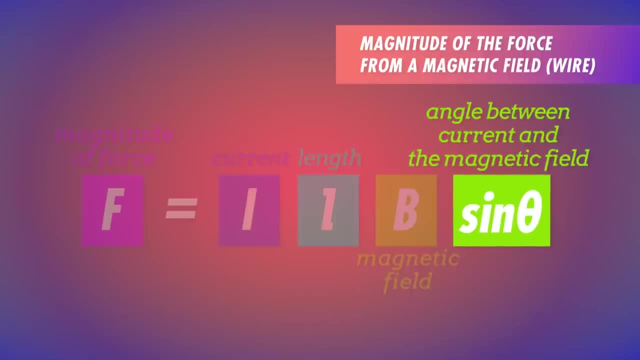 Currents are made up of moving electric charges, so it makes sense that a magnetic field would also exert a force on single electric charges that pass through it. And this is exactly what the Earth's magnetic field does to the charged particles coming from the Sun. It deflects them, sending them spiraling away and protecting us from the worst of the radiation. 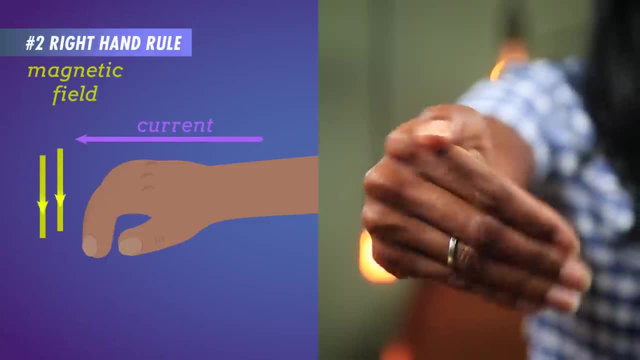 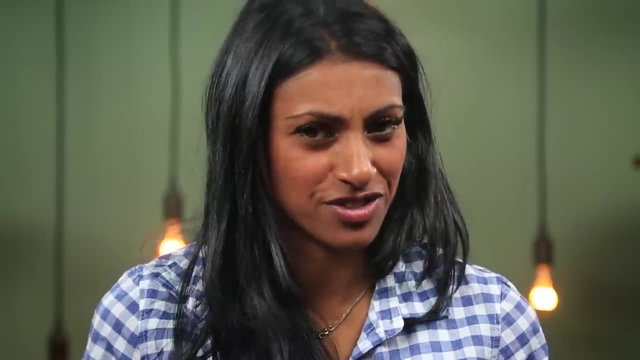 This represents the direction of the magnetic field. Your thumb, which is perpendicular to your fingers, is the direction of the force on the wire. But what about the strength of that force? You can use your hands to figure this out too, But you'll have to use them to do math. 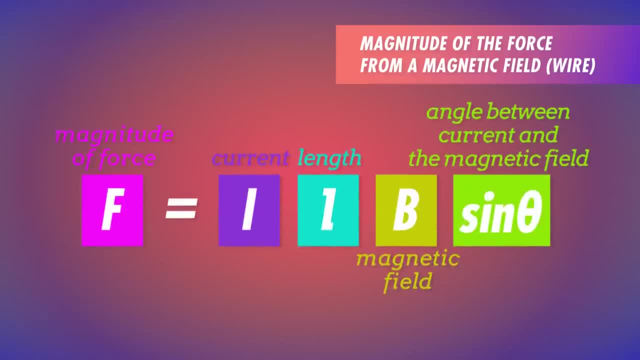 Sorry. The magnitude of the force from a magnetic field on a wire is equal to ilb sine theta. This equation tells us that there are four factors that affect the magnitude of the force. First, there's the current in the wire, That's i. 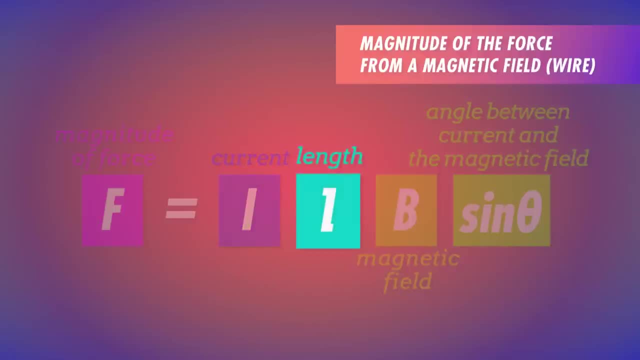 And the stronger it is, the stronger the force is. Second, there's the length of the wire running through the magnetic field, That's l, And the longer the wire is, the stronger the force is. Third, there's the magnetic field B. 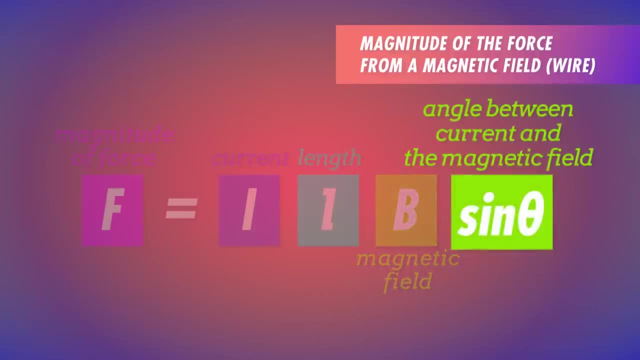 And the stronger B is, the stronger the force. Finally, the closer to perpendicular the current is with respect to the magnetic field's direction, the stronger the force is. That's where sine theta comes in. Its maximum value is one when theta is 90 degrees. 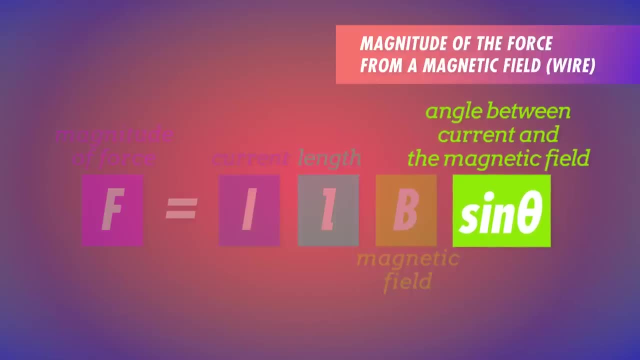 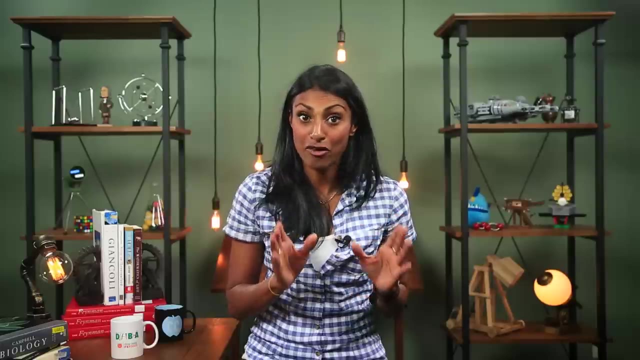 So the current is perpendicular to the magnetic field lines. That's when the force will be strongest. Similarly, the minimum value of sine theta is z zero when theta is zero. so that means the current is parallel to the magnetic field lines, and in that case there won't be any force on the wire at all. 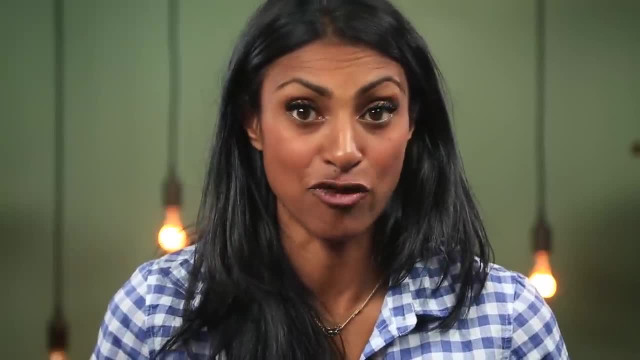 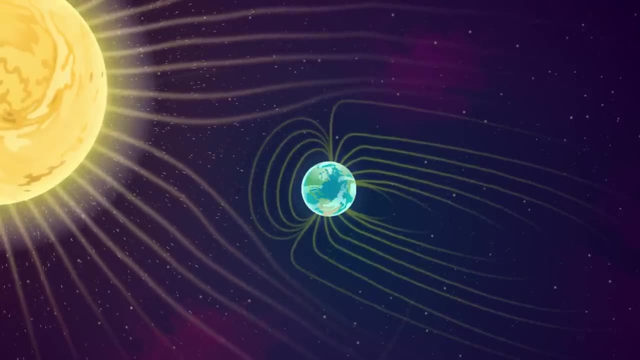 Now all of this math can help us understand how we're being protected right now from solar radiation. The Sun is constantly shooting radiation towards Earth in the form of charged particles, But luckily for us, Earth has a magnetic field. Currents are made up of moving electric charges, so it makes sense that a magnetic field would 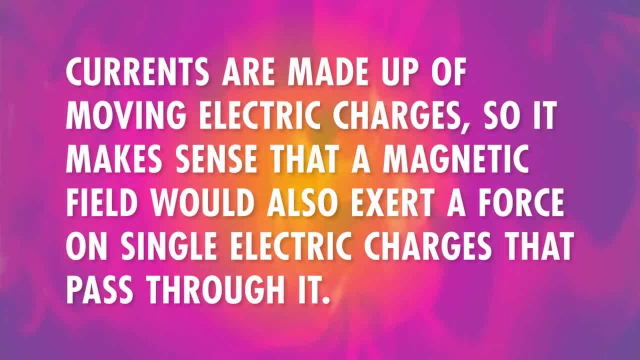 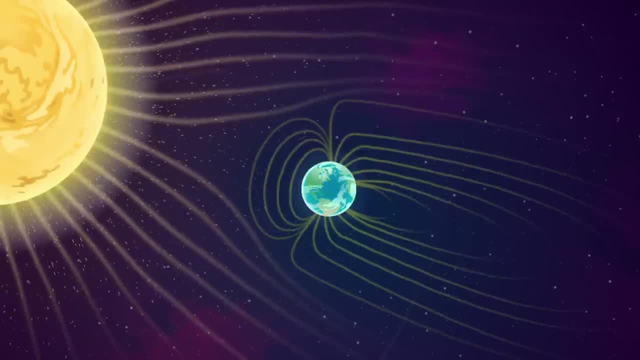 also exert a force on single electric charges that pass through it, And this is exactly what the Earth's magnetic field does to the charged particles coming from the Sun: It deflects them, sending them spiraling away and protecting us from the worst of the radiation. Let's suppose you wanted to find the magnitude of the force of the magnetic field on a single charged particle from the Sun. All you'd have to do is change the equation we use for the force on the current to account for the fact that we're talking about a single charge. 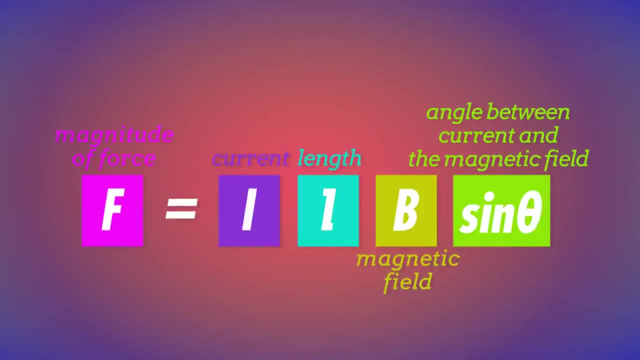 The equation for the force of a magnetic field on a current says that the strength of the force is equal to the current times, the length of the wire times the strength of the magnetic field times the sine of the angle between the current and the magnetic field. 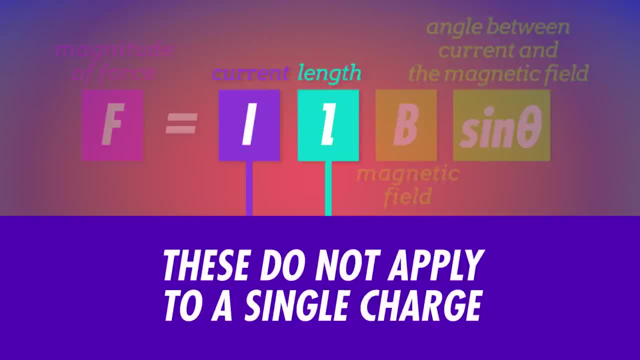 Now, two of those variables don't apply to a single charge – the current i and the length l. But current is just equal to the number of charged particles passing a given point over a certain amount of time, which we'll call n times their charge q divided by that. 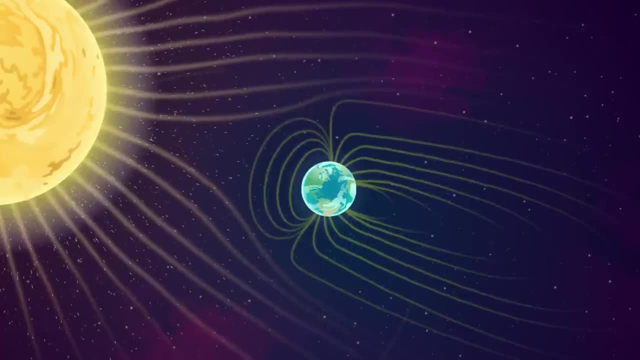 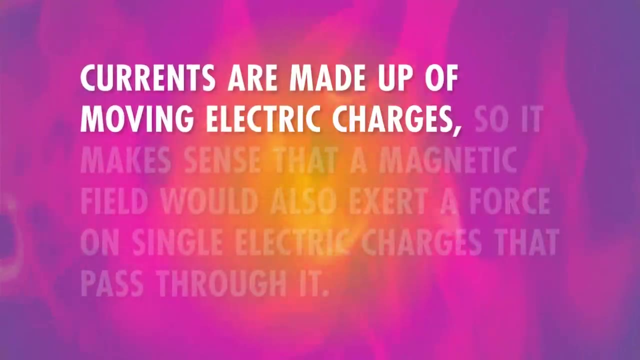 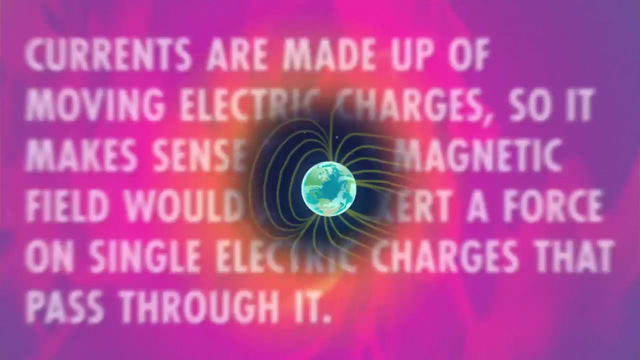 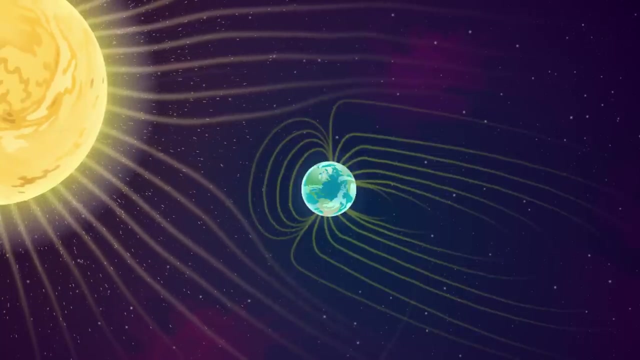 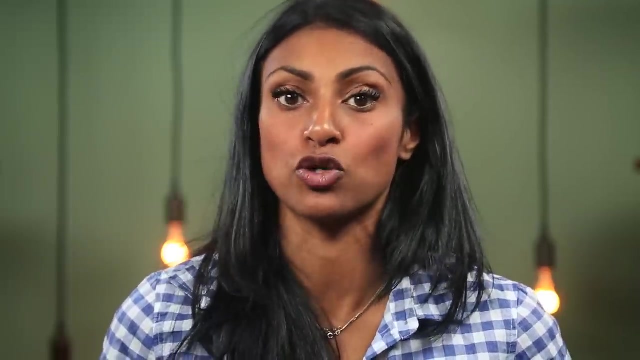 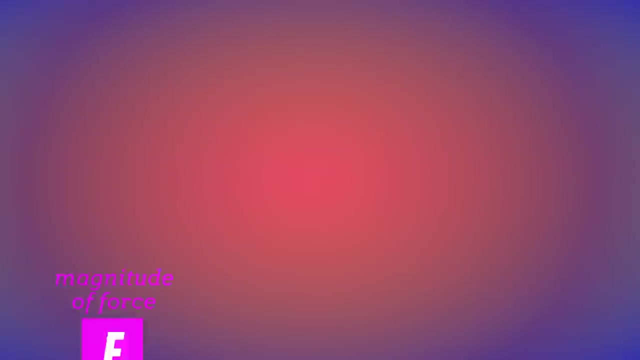 Let's suppose you wanted to find the magnitude of the force of the magnetic field on a single charged particle from the Sun. All you'd have to do is change the equation we use for the force on the current to account for the fact that we're talking about a single charge. The equation for the force of a magnetic field on a current says that the strength of the force is equal to the current times the length of the wire times the force. Times the strength of the magnetic field times the sine of the angle between the current and the magnetic field. Now, two of those variables don't apply to a single charge – the current, i, and the length, l. But current is just equal to the number of charged particles passing a given point over a certain amount of time, which we'll call n, times their charge, q, divided by that time, t. 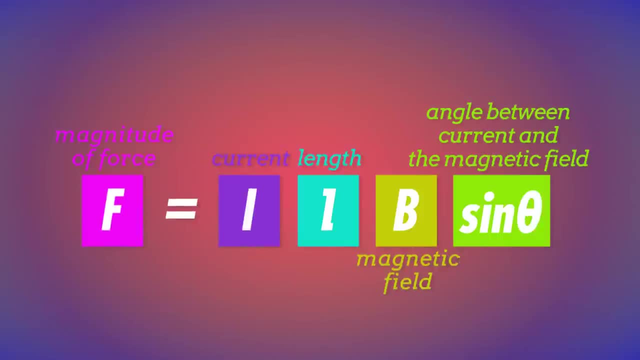 For a single charge, n is just 1, and the length is just equal to velocity, v, multiplied by time. So we can apply these two facts to our equation for force. 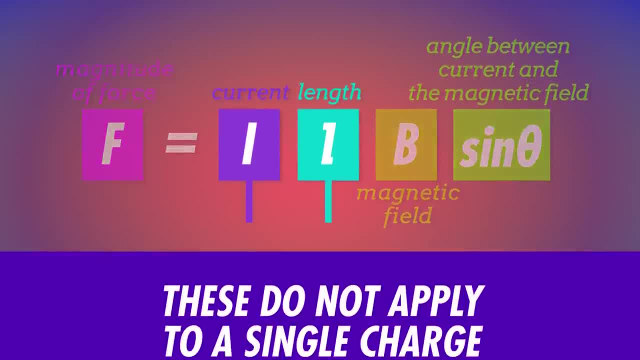 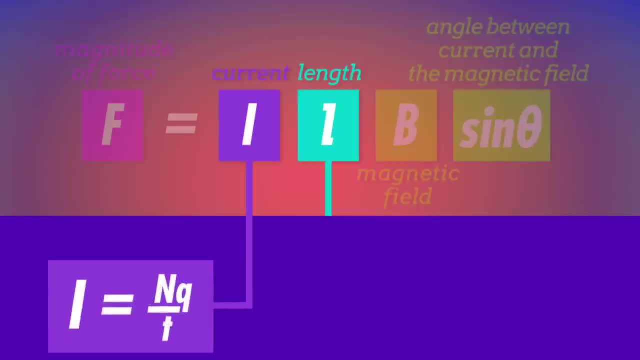 Which tells us that the force on an electric charge moving through a magnetic field is equal to q divided by time, multiplied by velocity times time, times the strength of the magnetic field, times the sine of theta. These two t's cancel each other out, so the equation simplifies to F equals qvb sine theta. 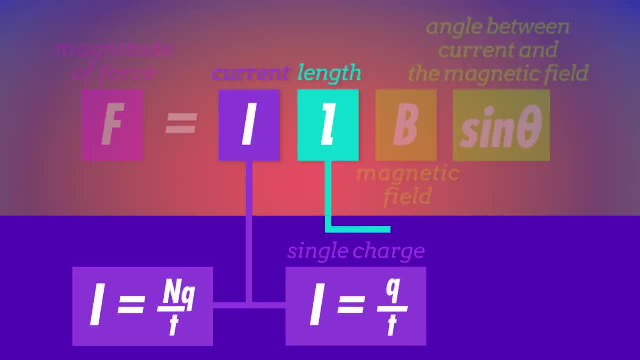 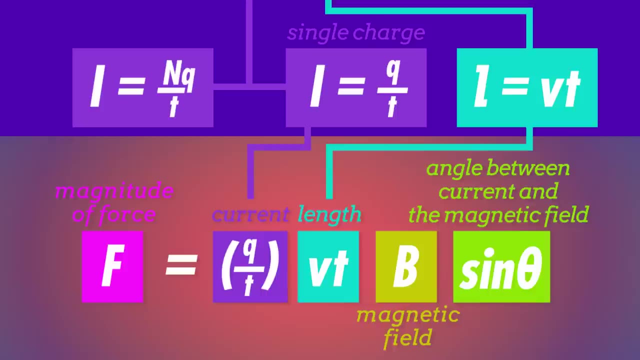 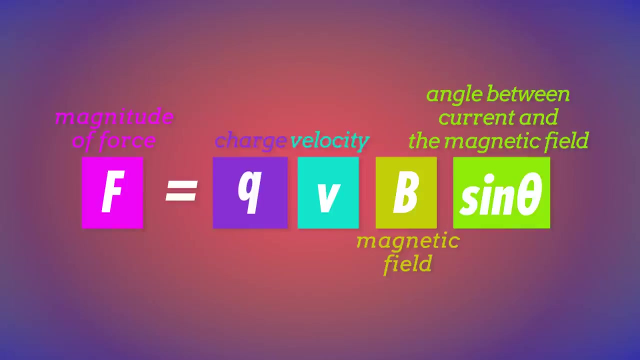 That means that, like the force on a current running through a wire, the force on a single electric charge depends on four factors. One is the same as with a current – the stronger the magnetic field, the stronger the force. The other three factors are slightly different from the case with a single charge. First, the force is stronger the closer to perpendicular the charge's velocity is to the magnetic field lines. Which means that if the charge's velocity is parallel to the magnetic field lines, there won't be any force on it whatsoever. 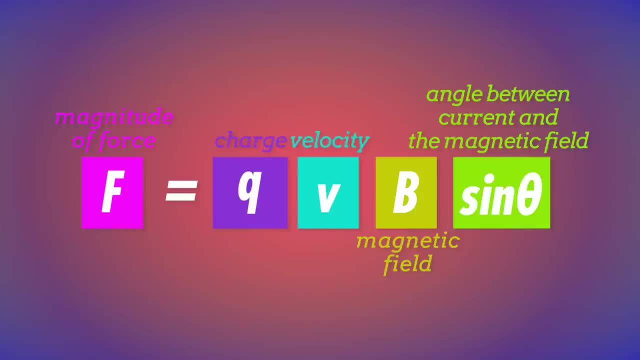 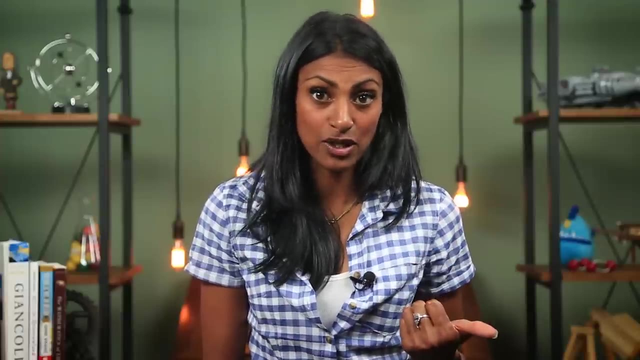 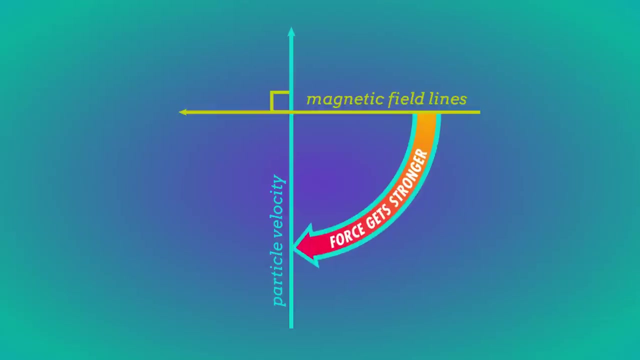 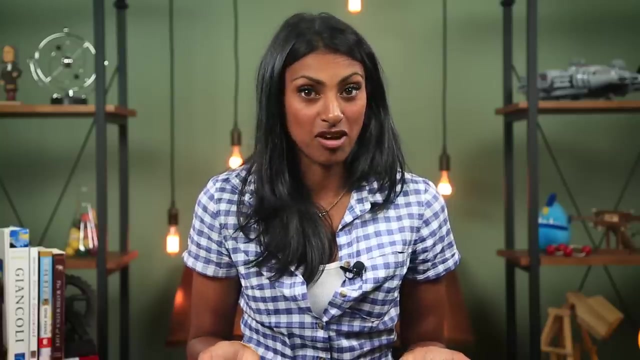 Second, the more charge the particle has, the stronger the force. And third, the faster the particle is moving, the stronger the force. Finding the direction of this force is where the third right-hand rule comes in. So get your right hand out again, straighten your fingers with your thumbs stretched outward. Then point your arm in the direction of the particle's direction. Then bend your fingers to make them point in the direction of the magnetic field lines. This is where things get a little tricky. If the charged particle is positive, your thumb is pointing in the direction of the force. But if it's negative, the force is pointing in the direction opposite your thumb. 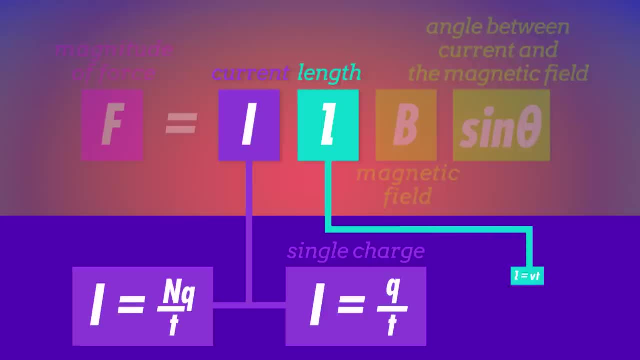 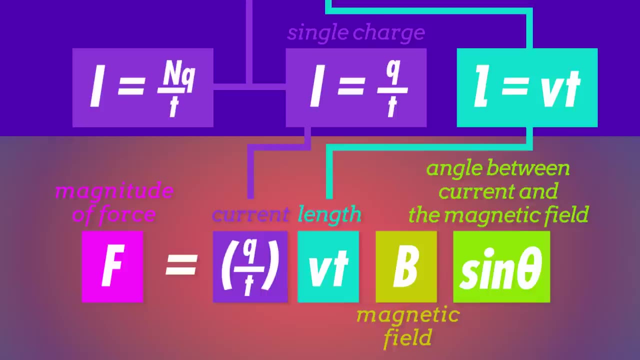 time t For a single charge, n is just one, and the length is just equal to velocity v multiplied by time. So we can apply these two facts to our equation for force, which tells us that the force on an electric charge moving through a magnetic field is equal to q divided by time multiplied. 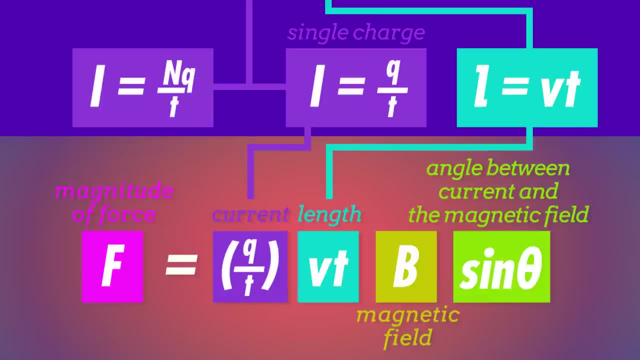 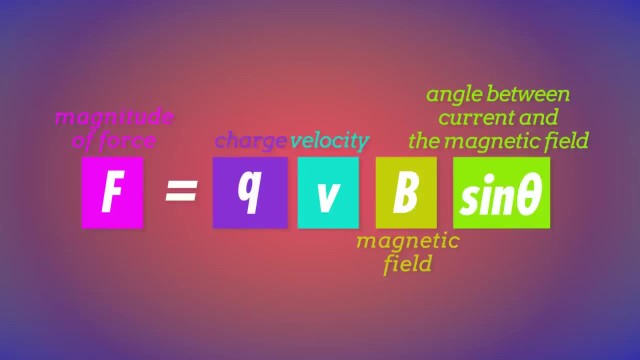 by velocity times, time times, the strength of the magnetic field times the sine of theta. These two t's cancel each other out. so the equation simplifies to: F equals qvb sine theta. That means that, like the force on a current running through a wire, the force on a single 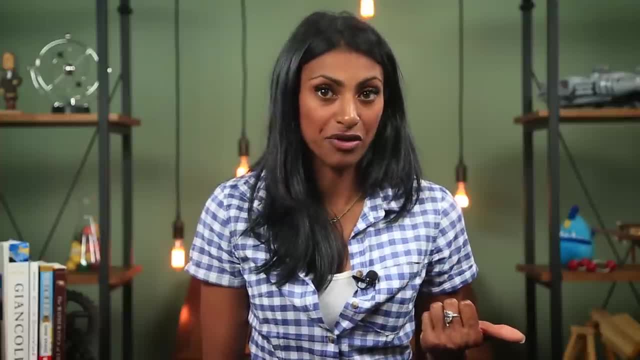 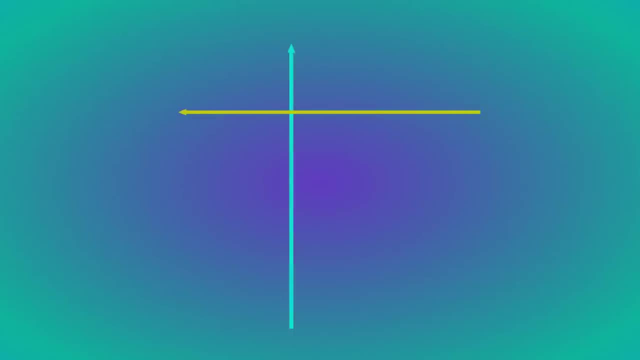 electric charge depends on four factors. One is the same as with a current – the stronger the magnetic field, the stronger the force. The other three factors are slightly different from the case with a current. First, the force is stronger, the closer to perpendicular the charge's velocity is. 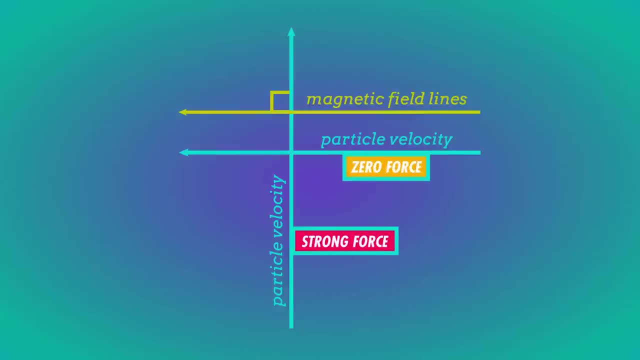 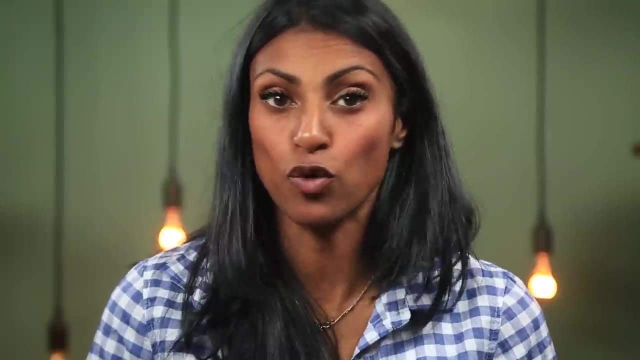 to the magnetic field lines, Which means that if the charge's velocity is parallel to the magnetic field lines, there won't be any force on it whatsoever. Second, the more charge the particle has, the stronger the force. And third, the faster the particle is moving, the stronger the force. 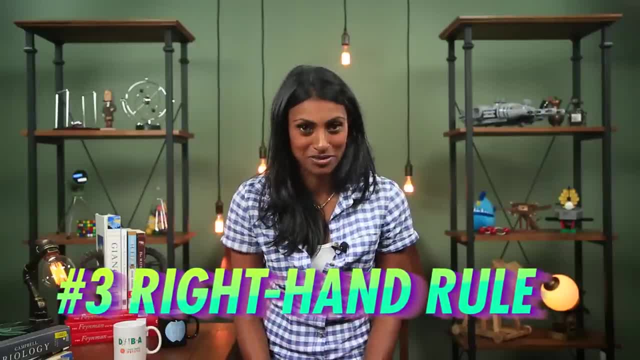 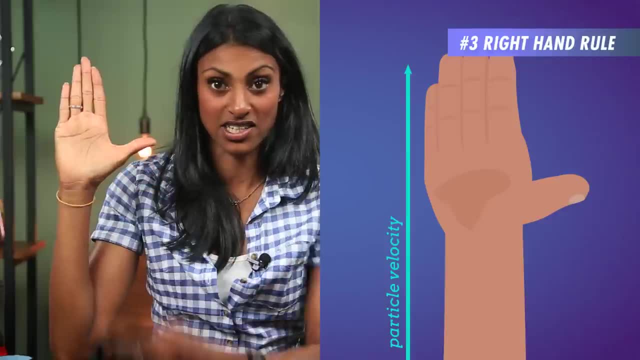 Finding the direction of this force is where the third right-hand rule comes in. So get your right hand out again. straighten your fingers with your thumbs stretched outward. then point your arm in the direction of the particle's velocity. Then bend your fingers to make them point in the direction of the magnetic field lines. 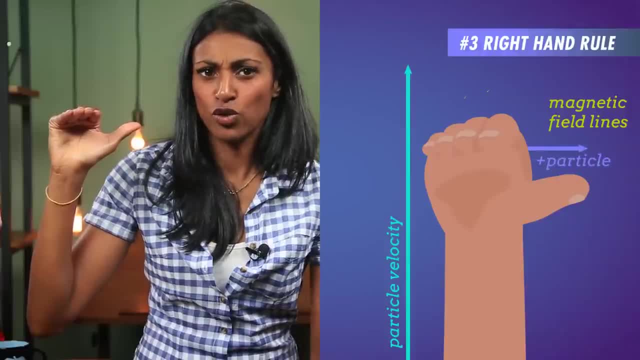 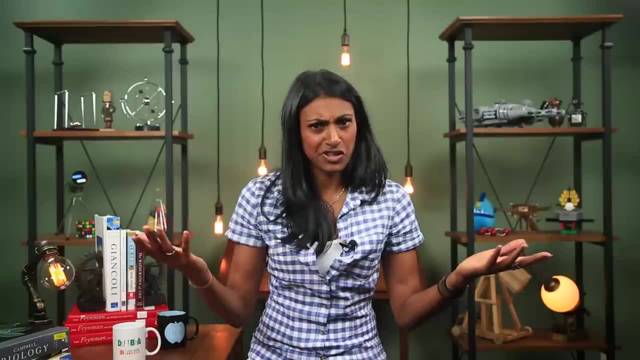 This is where things get a little tricky. If the charged particle is positive, your thumb is pointing in the direction of the force, But if it's negative, the force is pointing in the direction opposite your thumb. So electric currents create magnetic fields, and magnetic fields exert forces on electric. 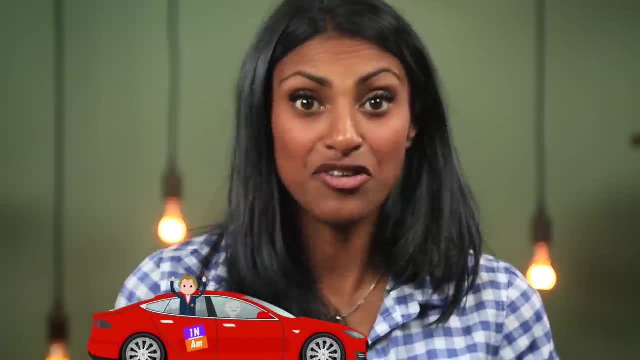 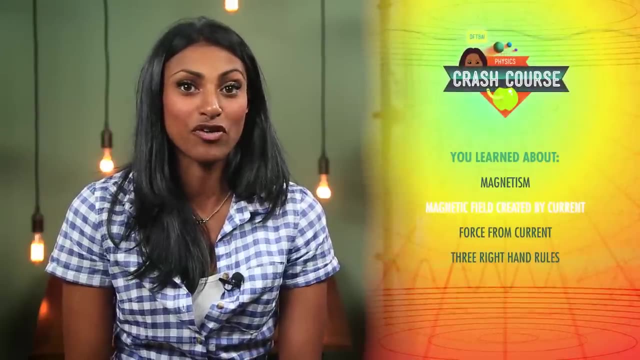 currents and charges. Oersted's experiment was simple, but his discovery linked two major fields of physics and inspired other scientists to do a lot more experimenting. Today you learned about magnetism and the magnetic field created by magnetic fields. We also talked about the force from a magnetic field on a current running through a wire. 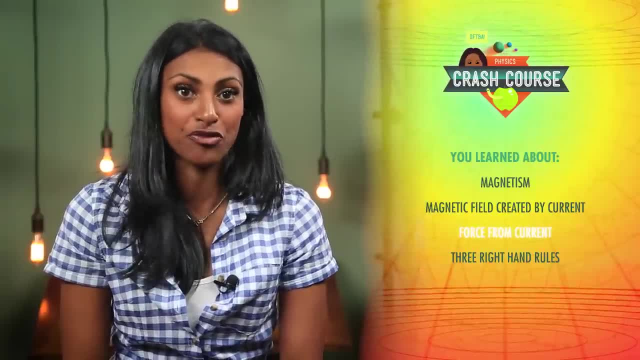 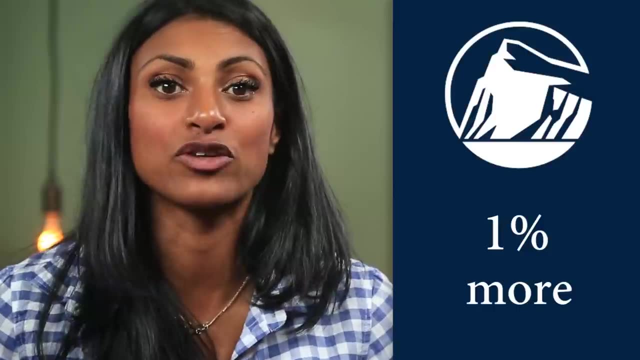 and on a single charge, moving through a magnetic field, And we went through the three right-hand rules. Thanks to Prudential for sponsoring this episode, Saving a little more today, even just 1% more of your annual income, can go a long way toward.